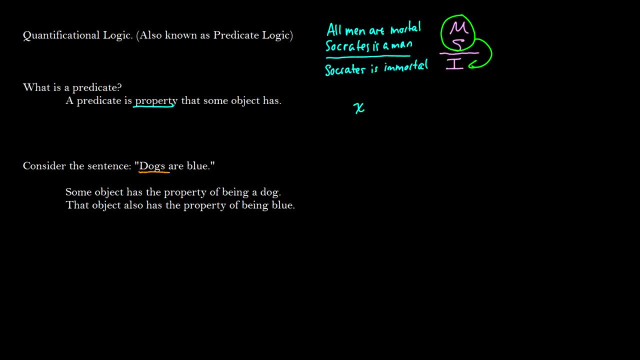 and we're going to have this sentence here: dogs are blue. Now, if we take an object and we want to capture the fact that dogs are blue with an object, this object is going to have the property of being a dog and it's also going to have the property of 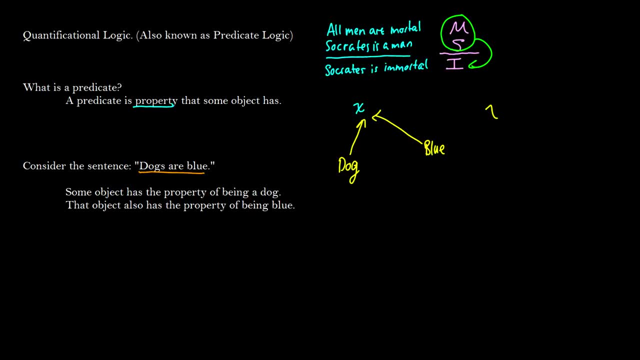 being blue. So we can say that this x is a blue dog. So this is what we mean by predicates. So, when we take this example, all men are mortal. Socrates is a man. therefore, Socrates is immortal. what we can say is that we have this random object x that has the property of being a man. 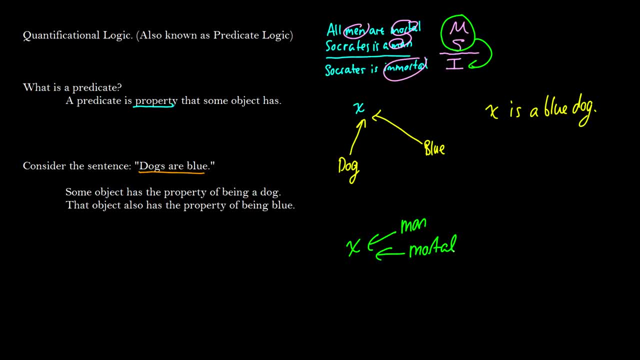 and has the property of being immortal. I totally wrote: Socrates is immortal, therefore Socrates is mortal. That's great. I wonder if anyone caught that. So now what we have is we say, okay, well, Socrates is a man, so we can write S, which is a man. Now what I should write is brackets here. 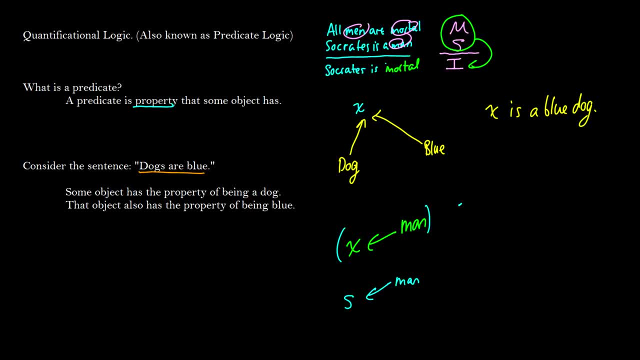 that if x is a man, then x is mortal. So we have this concept here, that S is a man. Therefore we can also claim that S is mortal. I didn't write this out properly yet, because I want to introduce the syntax first before writing out formal equations. 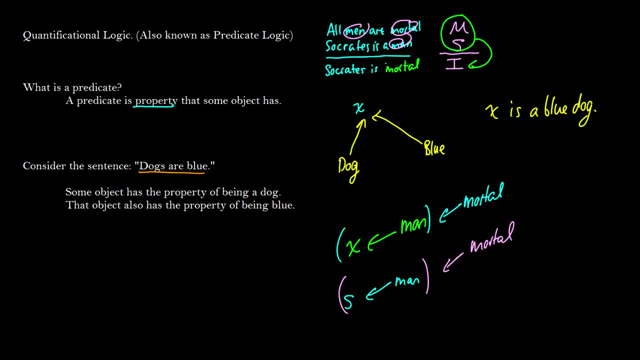 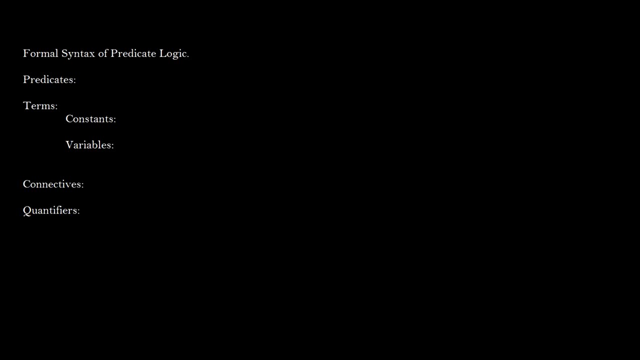 But this is the main idea. We can now break this argument up, our propositions, into arguments about properties, and we can extend properties. So let's talk about the syntax of formal logic. For predicates which are our properties, we will use capital letters. 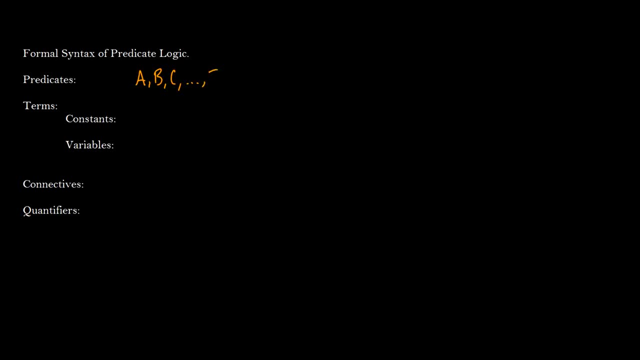 So a, b, c all the way to z, and we might even use a prime all the way to z prime. This is why I don't like using capital letters for sentences, because in predicates that's what we use for predicates universally. 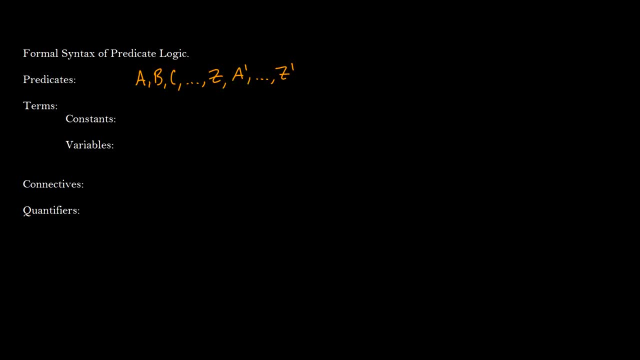 This is a universal thing As far as terms. terms are our abstract idea of an object, So we have constants which will be a, b, c, all the way up to probably t. I would say up to t is good. 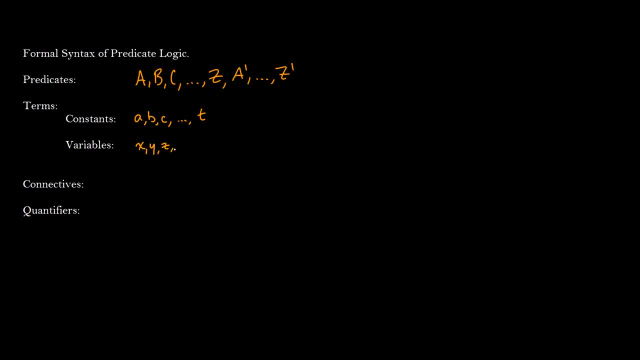 And our variables are going to be x, y, z, and occasionally we use w, u and v. So when we talk about specific properties, like when we said Socrates, for example, he would be a term, he would be a constant, he is not going to change. 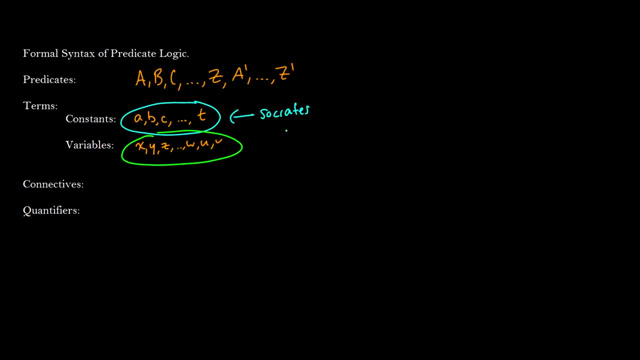 But when we talk about our variables here, what we just mean is some generic objects. We don't know which one it is. It's just some generic object that we haven't assigned any specifics to. We also have some connectives in our logic which are the same as before. 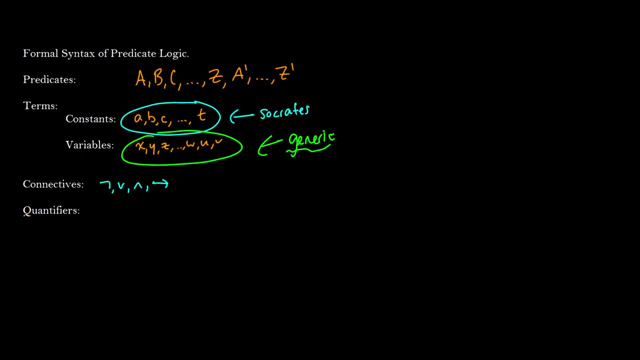 We have a negation or and a conditional- In fact, we also have the biconditional in here, if we want to include it- And now we have something new called quantifiers, And these are this upside down a which stands for all. 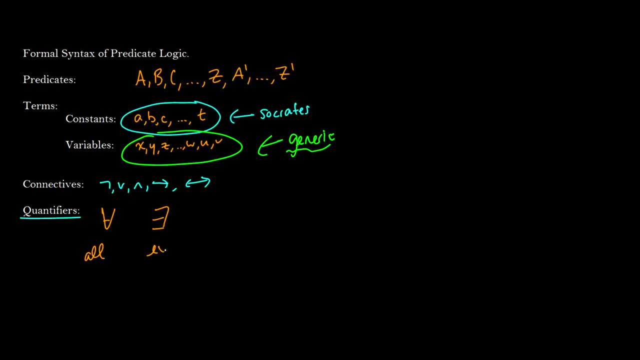 And we have this backwards e, which means exists. So if we want to say all x, we write upside down a. If we want to say there exists an x, we can write backwards e of an x. If we want to say all dogs are blue. 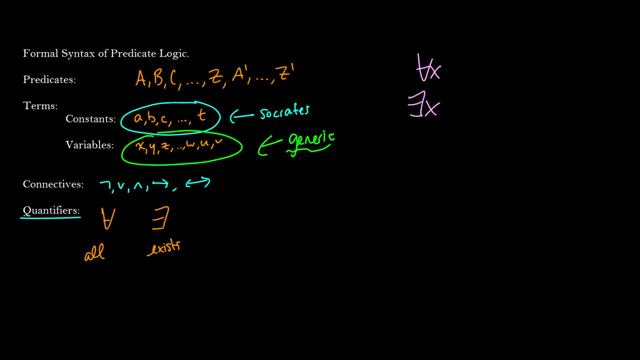 this is not correct logic, But if we want to understand how to use this new notation and what it means, as an example, all dogs- we can say all dogs, that's what the upside down means- are blue. And if you wanted to say some dogs are blue, 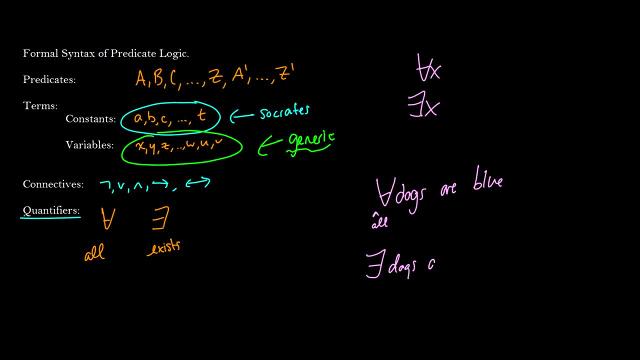 you can write this backwards: e Dogs are blue, So I guess a good thing would be some. That is a very good description of the existential. Of course this is not right. This is just a substitute, just to see exactly how you would use this. 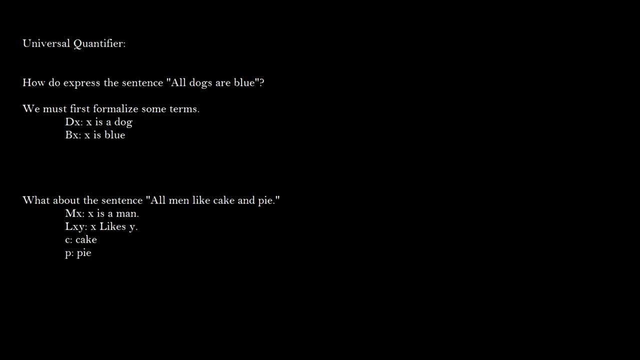 All right, Let's talk about the universal quantifier, the upside down a. Now how do we talk about the sentence all dogs are blue in our syntax, Well, we have to formalize some terms, So each predicate is going to be paired up with a variable. 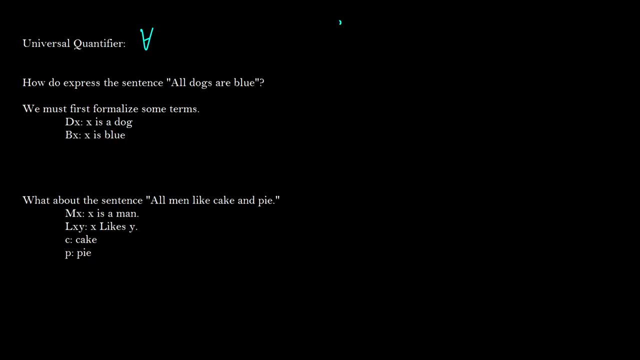 Kind of like an argument structure How you would say: oh, f of x is equal to y in math. You plug some x into f and then it spits out some value y. This is sort of what we're doing in here. 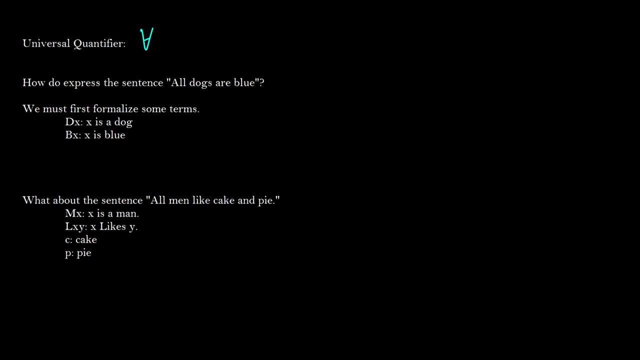 So we say dx means x is a dog. So dx means that some variable x is a dog. If we said, okay, what about d and fido? Then what that is saying is that fido is a dog Because fido has the property of being a dog. 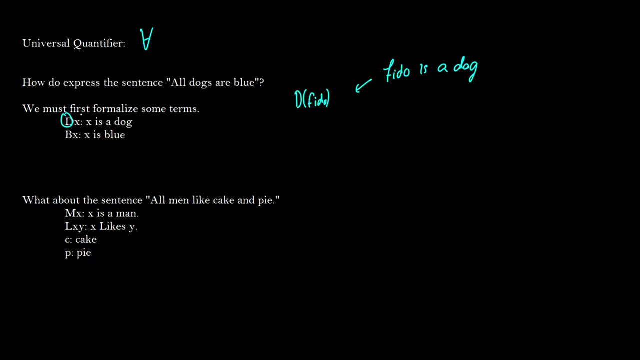 Where d here is the property and x is the thing that has that property. Now, what about x is blue? If we put b of fido in here, then we'd have fido is blue. So that's cool. What we do is we assign this variable to a property. 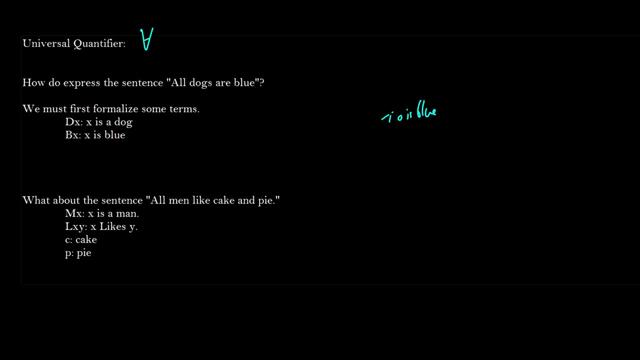 Now how do we write the sentence: all dogs are blue. Well, we're not talking about anything specific, So we need to use variables here. So, first of all, we have all- We didn't mean to write this upside down- a. 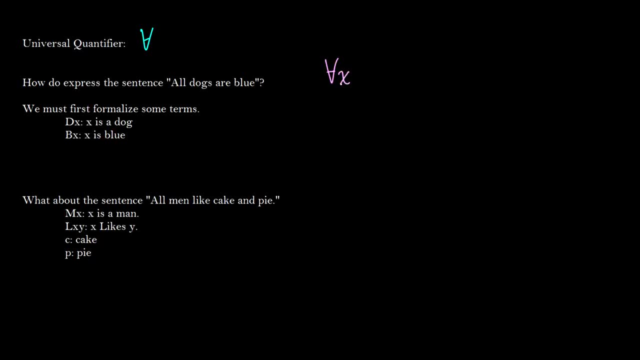 But what we want to say is all of some random or generic variable x. And now we want to say: for all x, if x is a dog, then x is blue. So this might be a little bit confusing, But we're taking an abstraction here. 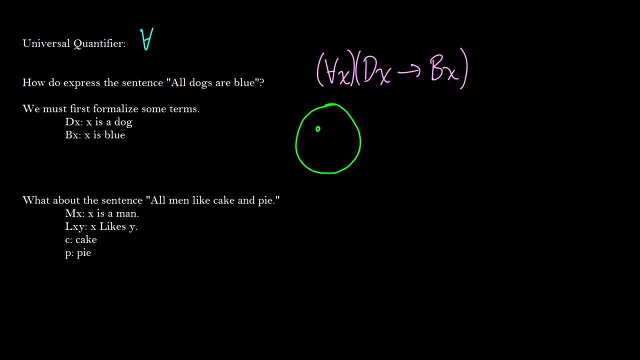 We're saying in this universe, if we pick a point x, so this is our lovely little universe right here, If we pick a point x and this x happens to be a dog, then we also know that it's going to be blue as well. 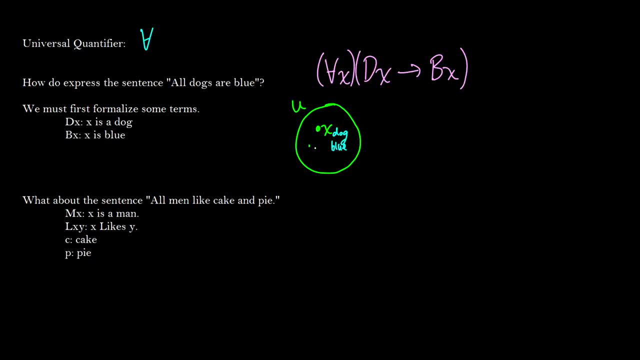 And it doesn't matter which x you pick in here. If it is a dog, then it's going to be blue, And this means that all dogs are blue, Because if you picked an x and it was a dog and it wasn't blue. 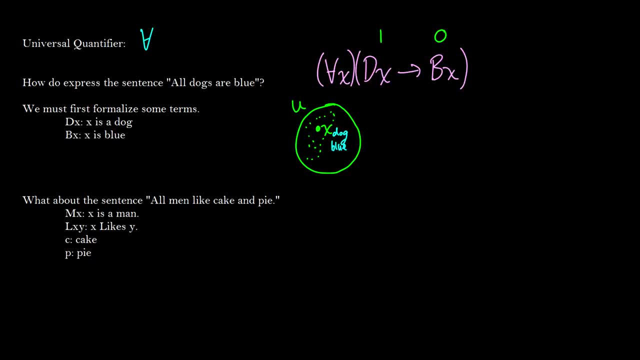 then it would be false, Because we would have the antecedent being true and the consequent being false, And we can't have that. So if the antecedent is true, then we guarantee that this consequent is true. 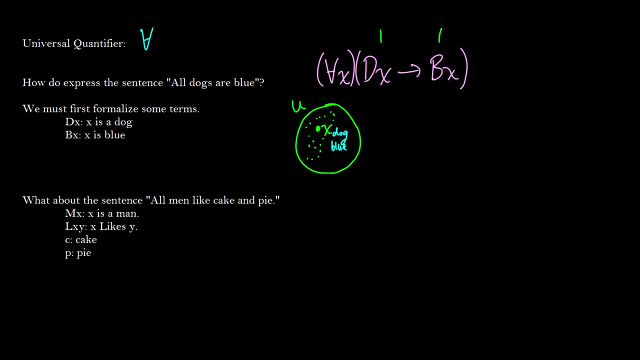 And that's what it means. So let's do a little bit more complicated example: All men like cake and pie. Well, the first part is fairly straightforward: For all x, if x is a man, and then we always use the arrow. 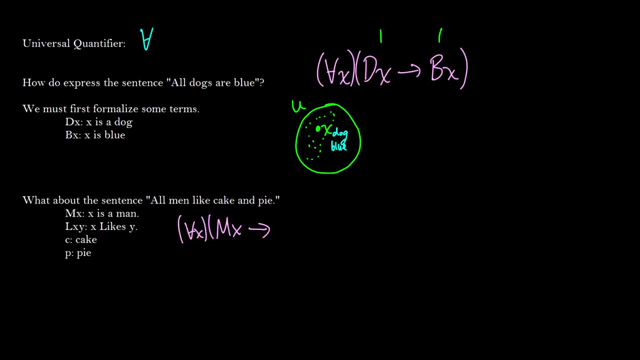 when we do universal quantifiers. I will explain this in a couple slides. don't worry, All men like cake and pie. Well, we have this new verb here that takes two variables. So when we write lxy, this translates as x likes y. 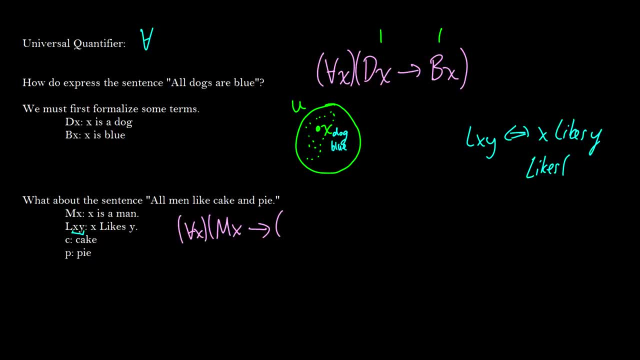 In fact, you can kind of write this as a function of likes, comma xy, So we can think of: men like cake. Well, x is a man, So for liking, x is going to like cake, which we've listed as c. 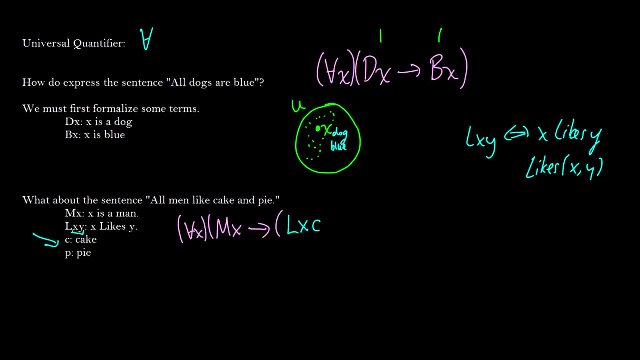 We don't need the property of x being a cake here, because we're talking about one specific thing. So we don't need to write in cx where x is a cake. We just take it as: oh, this occurrence is just cake. 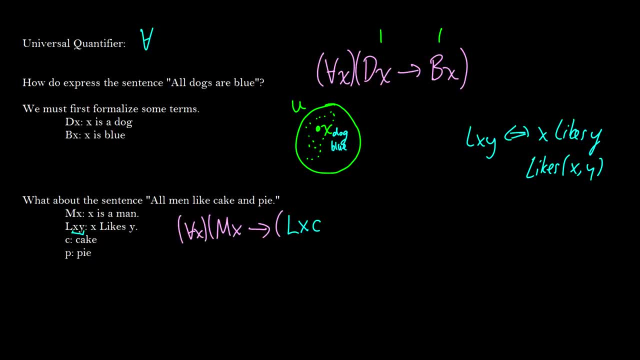 It is a constant. So we have all x. if x is a man, then x- this man likes cake and x also likes p. So we can write a sentence like this: For all x if x is a man. 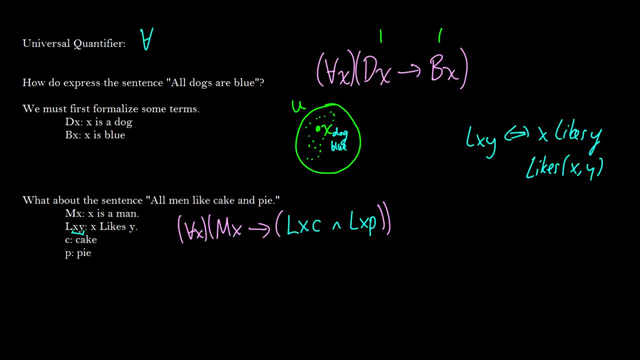 then x likes cake and x likes p, So this notation is something you have to get used to. But remember we're assigning property to these variables And these properties will stick with the variable until the variable gets outside the scope of this quantifier. 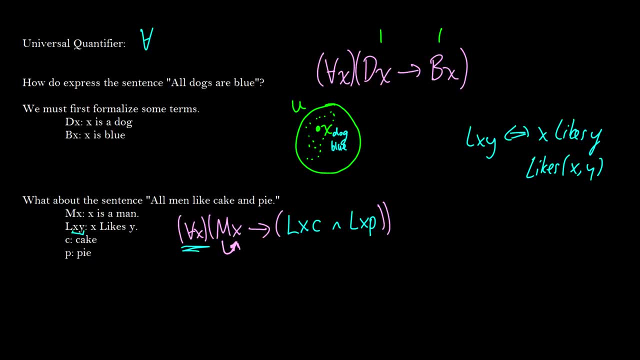 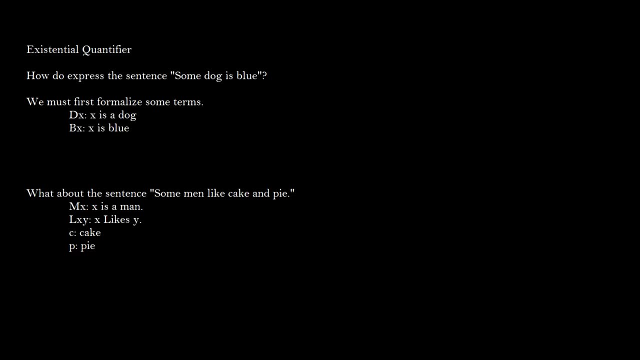 which we'll talk about a little bit later. Now we're going to do the same sentences with the existential quantifier. So before we had all dogs are blue, which was for all x. if x is a dog, then x is blue. 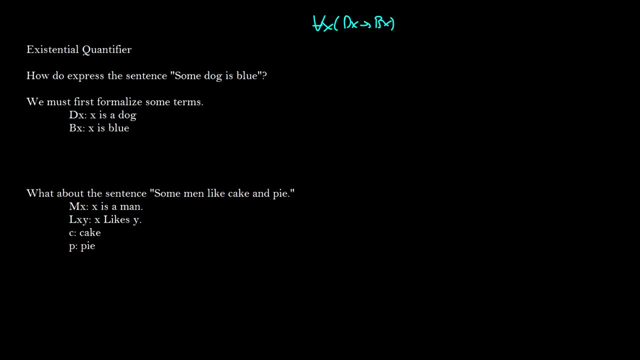 Now we want to say: some dog is blue, So we say there exists an x such that x is a dog. But here's the thing that's different With existential quantifiers we use: and So x is a dog. 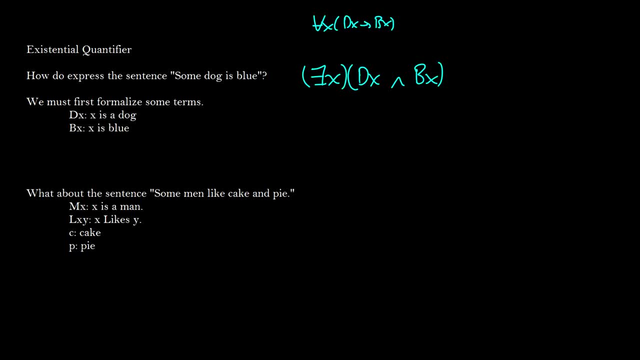 and x is blue. We're going to go over this in the next slide, But we use an and because there are some things that are just blue and there are some things that are just dogs, and there are also things that are dogs that are blue. 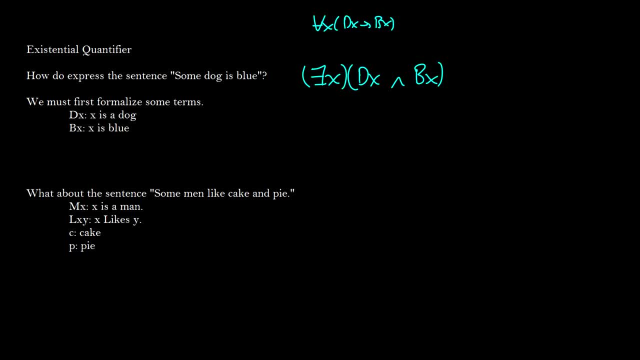 So we don't want to say that if x is a dog, then x is blue, because that would mean you can't have a dog that isn't blue. But if we say some dog is blue, there's also clearly going to be dogs that are black. 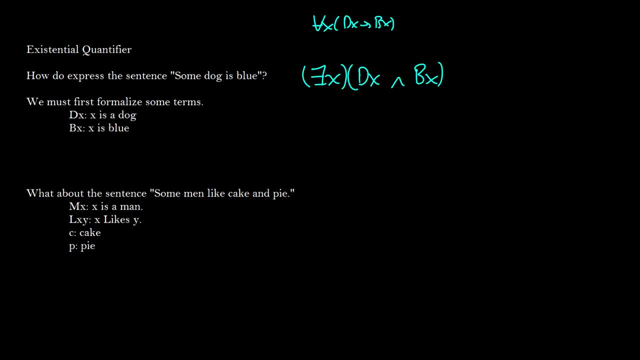 dogs that are red, dogs that are gray, and we don't want to have to capture all of those and have contradictions with our logic. So let's try some men like cake and pie. Okay, this is the same thing as before. 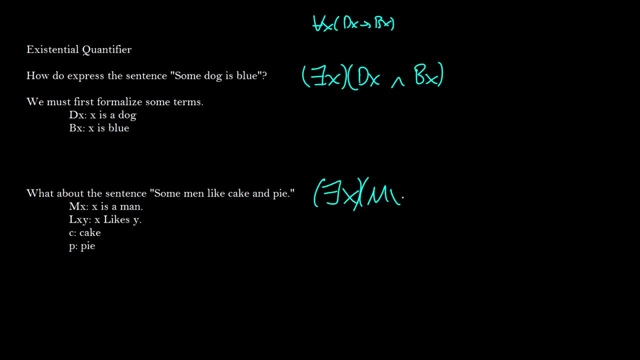 We say there exists an x, such that x is a man. okay, and this x likes cake and this x likes pie, So it's not too bad. It kind of makes sense, Hopefully. Now let's talk about why we use these specific connectives. 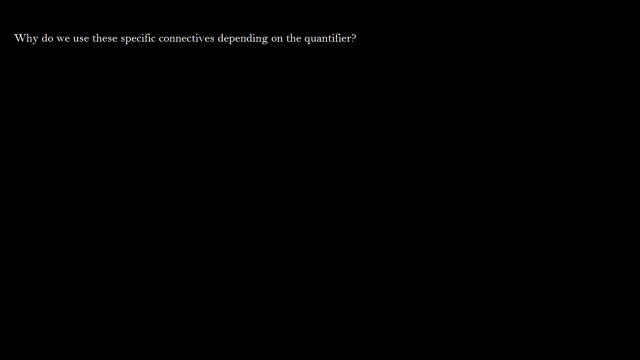 and I'm going to use some pictures here, because I think pictures help a lot. So here's the thing: We have this universe and I'm going to write some names of people- Mary, John and Steve- And we're going to assign these properties. 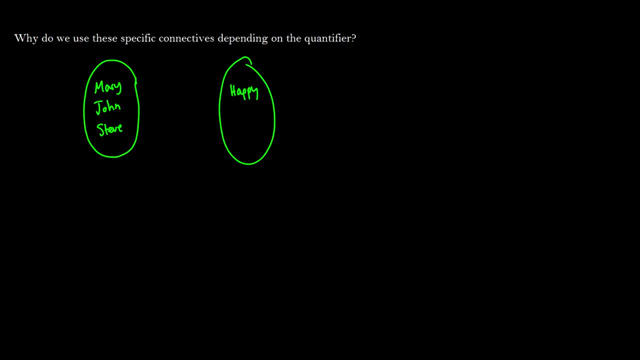 of being happy and being sad. So here's what we're going to say. We're going to say: Mary is happy, John is sad and Steve is happy. I'm going to make Mary a dude, So we're going to call him Mark. 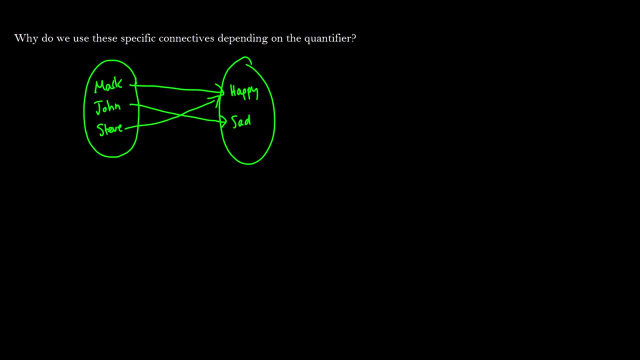 for the sake of example. Now, what we want to say is: all men are happy. So there's two ways we can write this: All x, mx, arrow hx, and for all x, mx and hx. Okay, 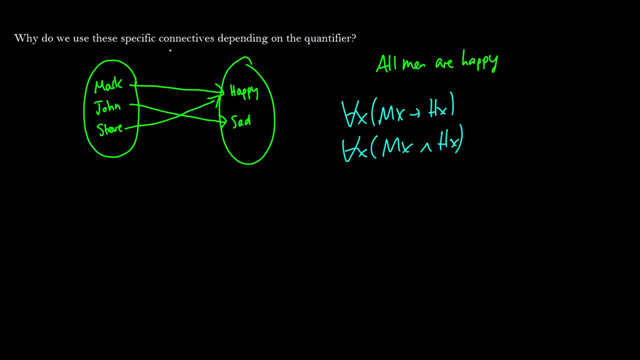 so, first of all, well, everyone here is an x or everyone here is a man, so we can write this antecedent: true? Are all of them happy? Well, there's one case where John isn't happy, so this will be false. 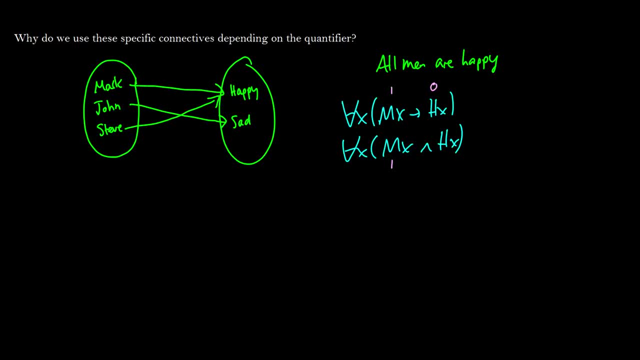 And in the second one there's a case where x is also not happy, so this is false. So in both cases, these are going to be false, which is fine. However, let's consider something a little bit different. 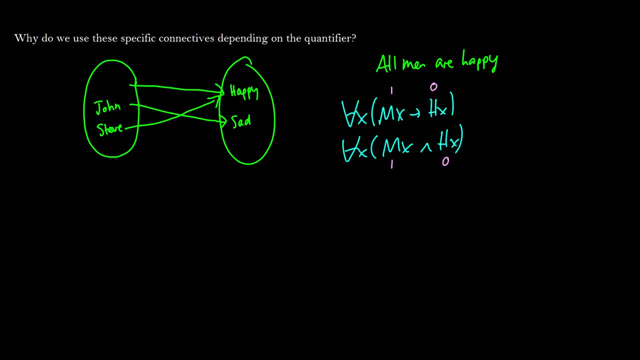 What if we change Mark back to a woman, Mary, Well, Mary's happy. I actually shouldn't change this one. I want to put this one back to Mark. I'm going to change Steve to a woman. We're going to make him Stacy. 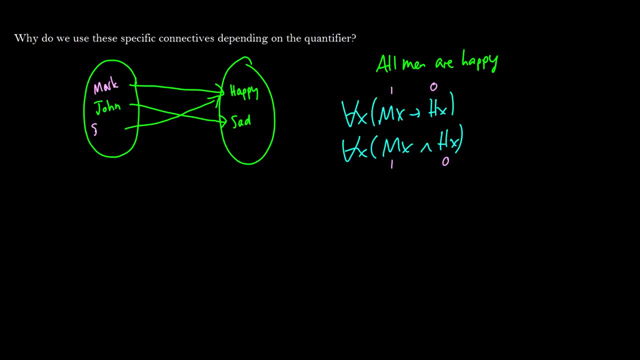 Okay. Do I want Stacy changed? No, I don't want Stacy changed. Why do I keep changing the wrong one? This is Steve. John is going to be, uh, Jocelyn. That's the best J name I can do. 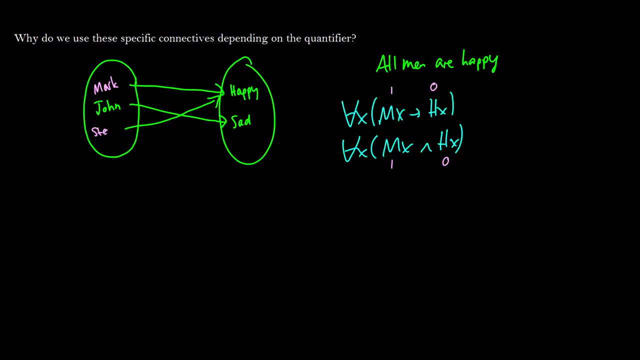 Okay, So this is Steve John is going to be- uh, Jocelyn, That's the best J name I can do. Okay, So this is Steve John is going to be- uh, Jocelyn, That's the best J name I can do. 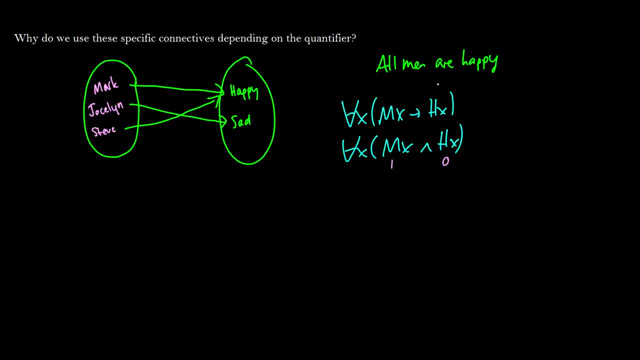 Okay, Now, in this case, not all X's are men, So this first part's going to be false, Because we have Jocelyn here, who is a woman. But are all men happy? Yes, All men are happy. 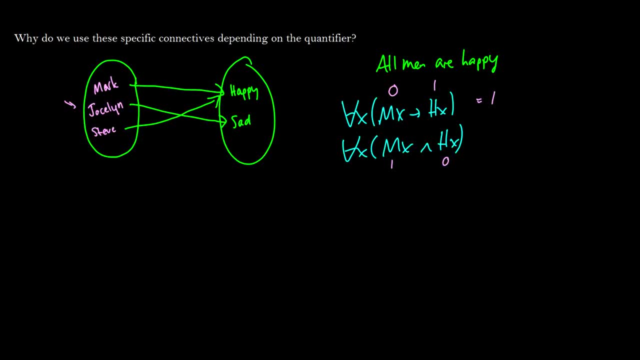 So this first part's going to be true. However, in the second part, it is true that all men are happy in this example, But is every element that we're looking at a man And 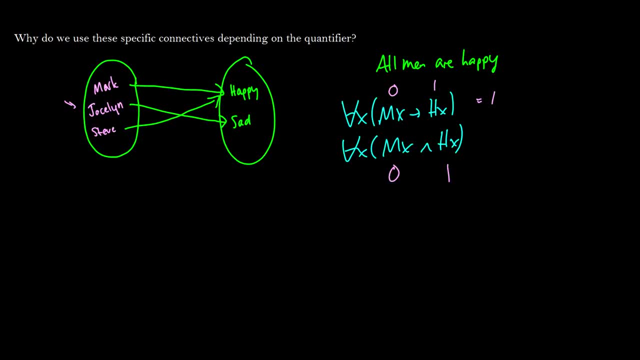 the answer is no. They're not all men. Therefore, this second one we have is false. But we know intuitively that all the men here are happy, Because Mark is happy and Steve is happy. But 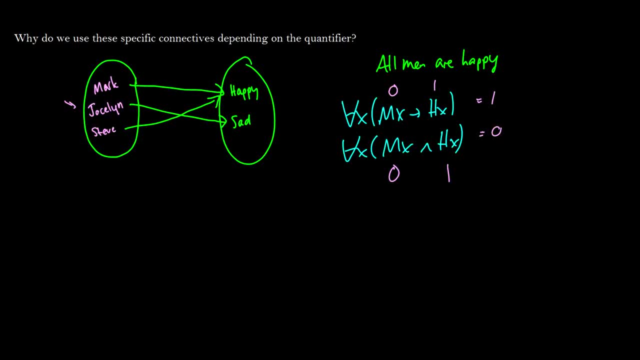 the way that quantification logic works is that when we have all X, Mx and Hx, we need to check: okay, is everyone a man? And if the answer is no, then it's going to be false. 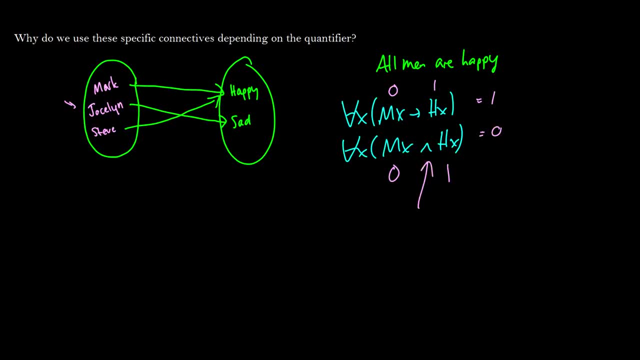 because of the requirements of the AND. So this is why we use the arrow for our universal quantifiers. Let's do the same thing, but let's take a look with the existential. okay, let's copy and paste that. 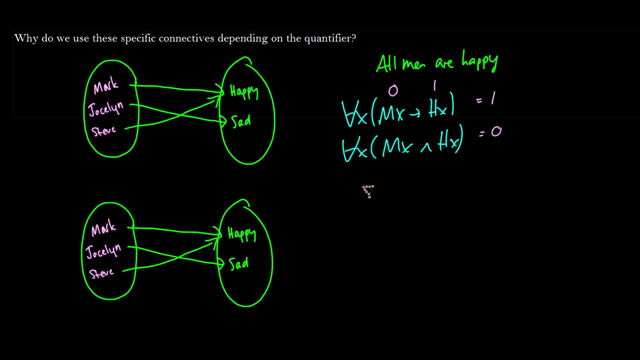 and we want to write. we want to write a sentence: like some man is happy. Okay, so we have. there exists an X such that Mx arrow Hx. and there exists an X such that: 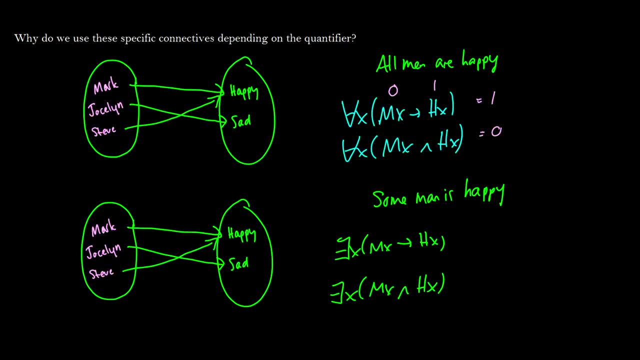 Mx and Hx. Okay, well, in our second example, it's clear that, yes, there is some person who's a man and there is some person that is a man that is happy. Okay. 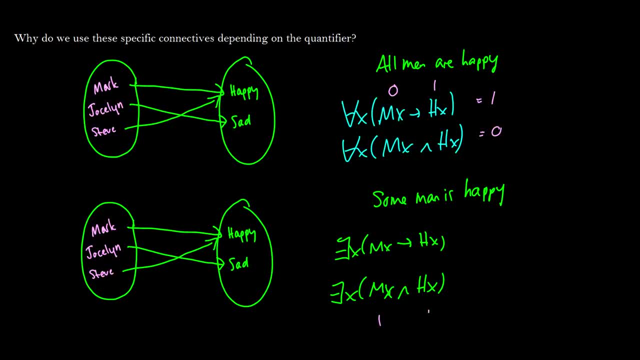 perfect. The bottom one is fine, However, the top one okay. X is a man. yes, there is some person who's a man and happy, So this also equals one. So both of them are good.